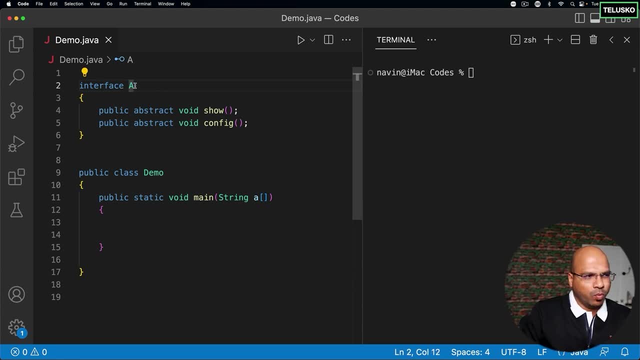 So let's understand that. So we have the interface a. Now you will say what is changing there. Now, first of all, interface is not a class. Okay, so that's why that's the main difference between abstract class and interface, And by default, every method in the interface is public, abstract. 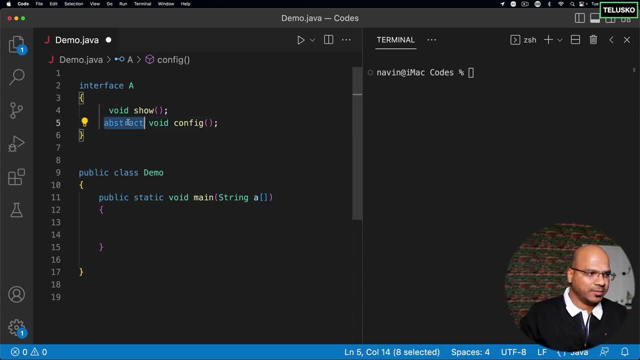 So these two keywords are actually not required because anyway they are public abstract. So even if you don't mention, they are by default public abstract and that's why, if you can see, when I put a semicolon just after the method, there is no error, because behind the scene, public abstract is there. 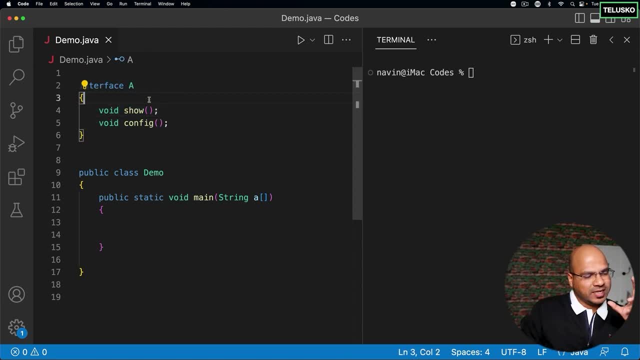 Now, this is your interface. So interface basically means it's like a class, just that all the methods are, by default, public, public, abstract. okay, but then how will I use this? how will I instantiate this? the same problem was there with abstract class. right, we cannot instantiate it. now, if you look at this, how do 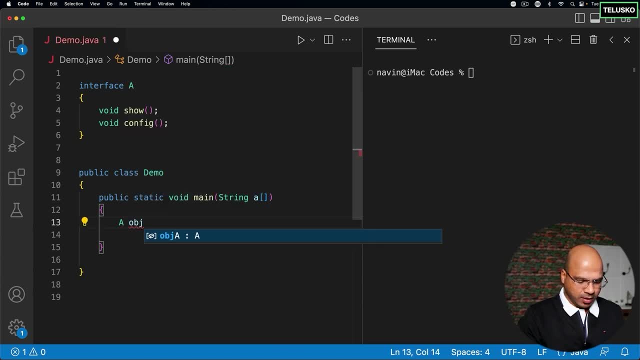 I instantiate, let's try. so I will say a obj. see, there is no problem in creating a reference of it. so that also means we are creating a type, the way you create classes. so let's say, if a is a class, you can say a obj. so a is a type, right. in the same way here the interface: a is a type, okay. 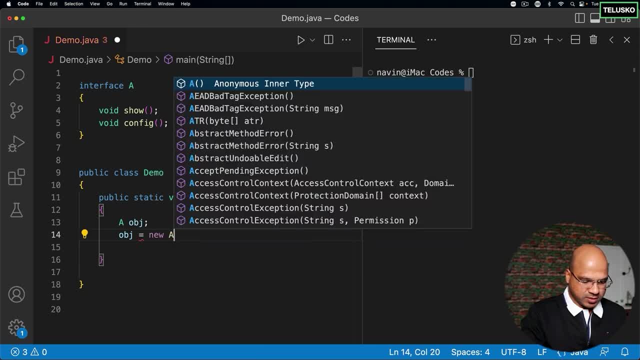 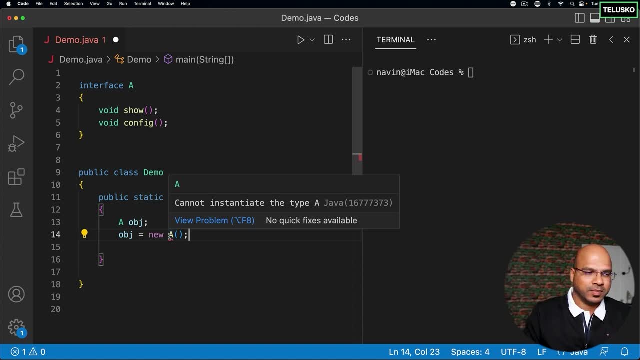 this works, but the moment you try to create object for this, it will give you an error. it says: if you see the error, it says: cannot instantiate the type a because it's interface. you can't instantiate it. okay, now what's the solution? the solution is: see first of all, why do we get interface? we get: 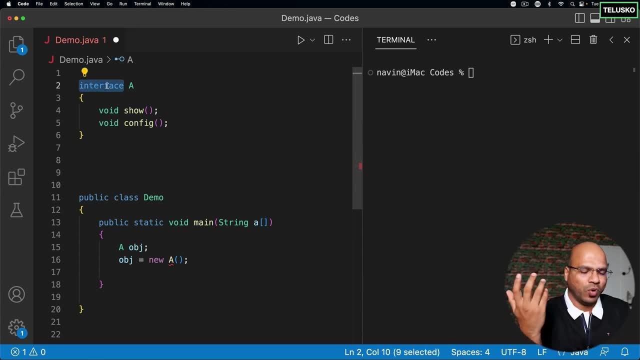 interface so that we can design something. we can say: example. let's say, if you ask me about how do we create a table, I can say: or maybe if you ask me how to read somewhere so I can say: go straight, take a right, go straight, take a right. take an Auto, take a bus, get down at the next stop. so what I'm? 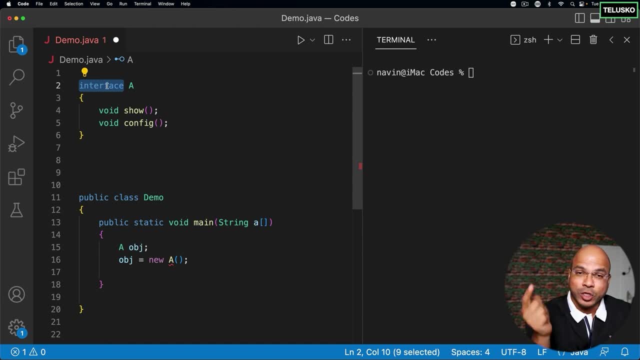 doing is: I'm giving you the path right. I'm giving your design. you have to literally take a walk. I will not walk for you, I will just show the directions. in the same way, interface says I will tell you what are the methods you need, but I will not implement them. it is your job to implement. 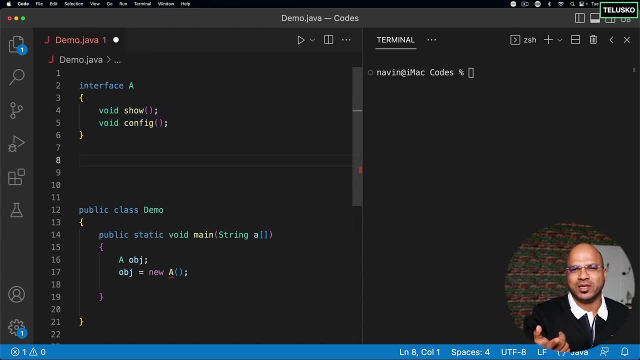 so when I say your, now I'm talking about classes. see, ultimately you create object of a class interface. just show you what you consider to be the object of a class, and so I'm giving you, your, you, the design. so here what I can do is I can create a class, let's say class B, so we have a. 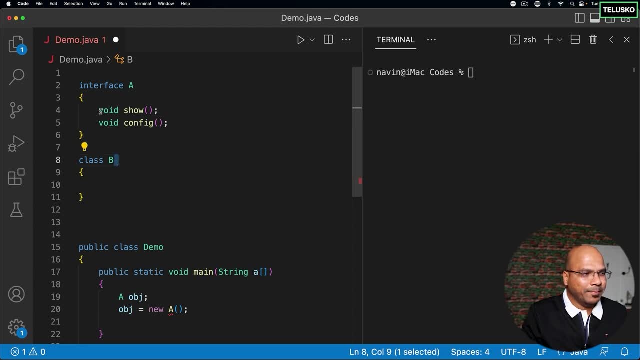 class B here and then in this class. I want to implement these two methods now. in terms of abstract class, we say extends- right, because class extends another class. here, A is the interface. we have to use a different keyword here. the keyword which we use is implements. so whenever you want, 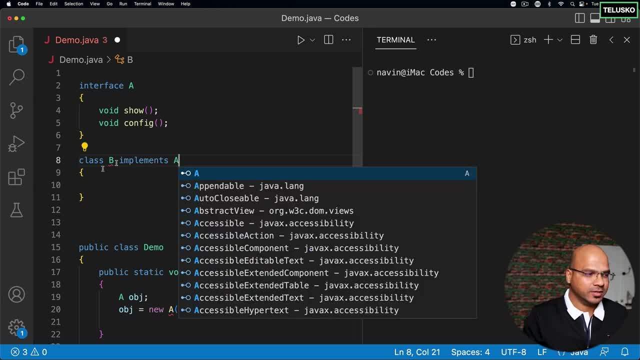 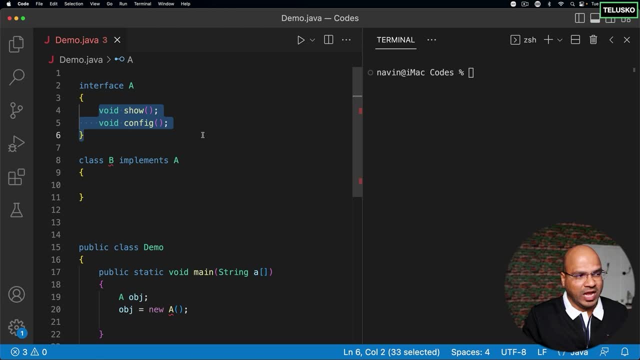 to implement the interface. you say implements keyword, and when you say implements, it becomes compulsory for you to define both the methods. okay, if you fail to define both the methods by default, your class also becomes abstract. okay, but we don't want to get abstract class right, we want. 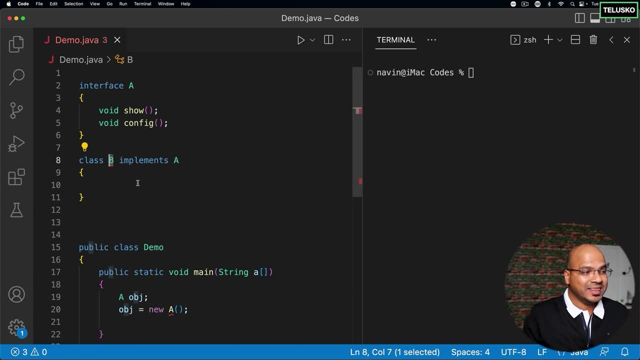 to create a concrete class. we want to create object of B. in that case it's your job to define both the methods. okay, there's one way you can use a shortcut here. you can just go back here and say: quick fix, it will ask you to implement the methods, or you can do the hard work. you can say: public void. 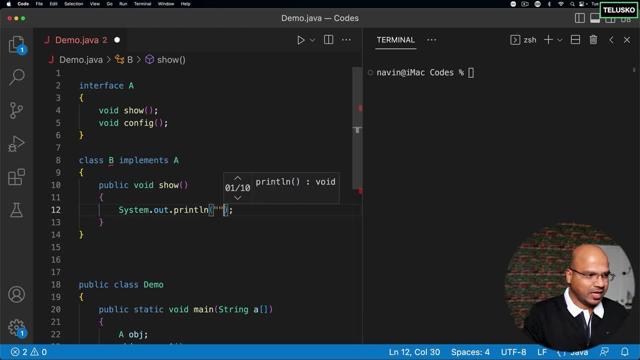 show, and then you can define something. here I can say: I'm defining in show and then we can define another method as well, which is config or public void config, and here we can define in config. so basically what you're doing is you are implementing both the methods, as I mentioned before. if you 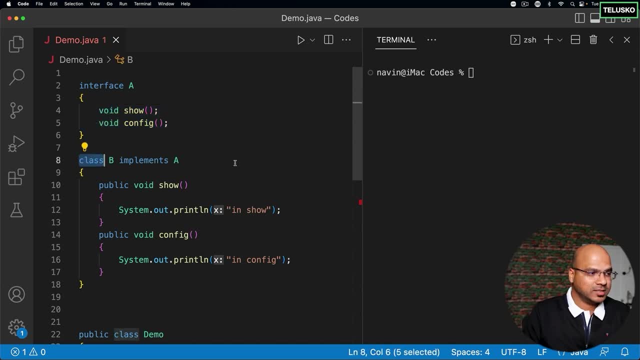 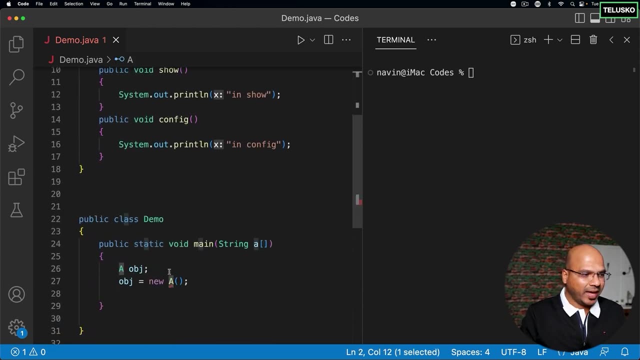 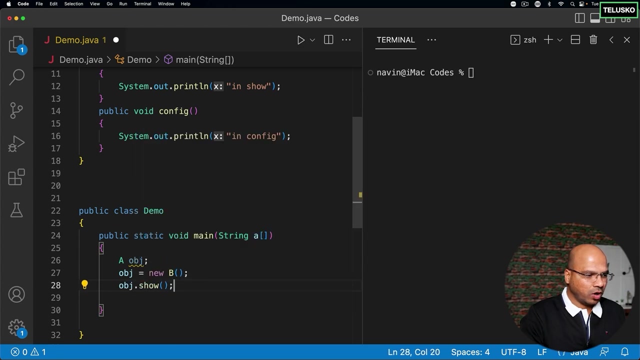 fail to implement these methods, or this class becomes an abstract class, but we are implementing it right now. when you implement, basically you can't create object of A, but you can create object of B and you can say it works. and now, using this obj, I can call show, I can call. 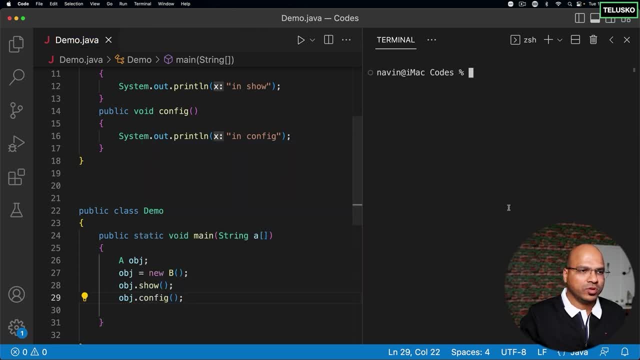 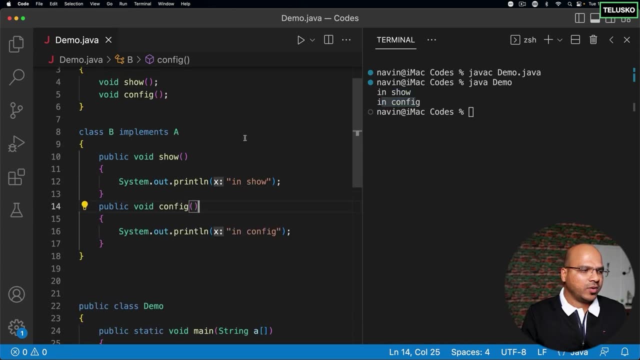 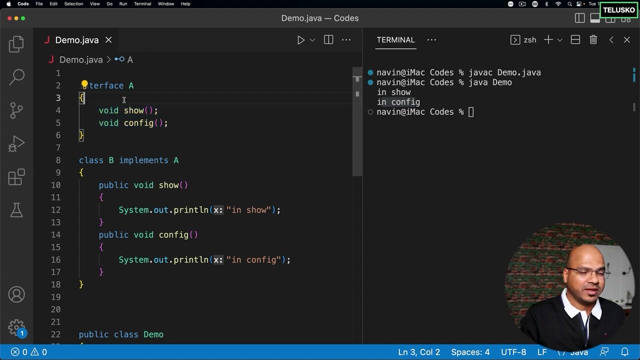 what other method we have. we have config, so we can call both the methods and that perfectly works. if I compile and run this code, you can see it says in show in config. okay, what else can I have? so the way you create variables here, also the way you create methods here can I create variables. 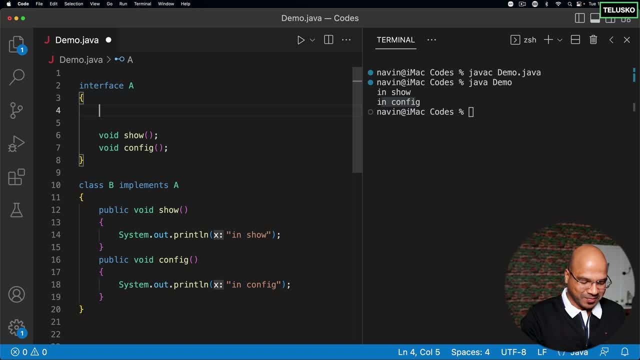 now. first of all, we don't define variables right, we declare them, so we can actually. so if I say int, let's say age, that's a variable. I know, I don't know why I'm taking this age variable every time, but let's say we have int age here. 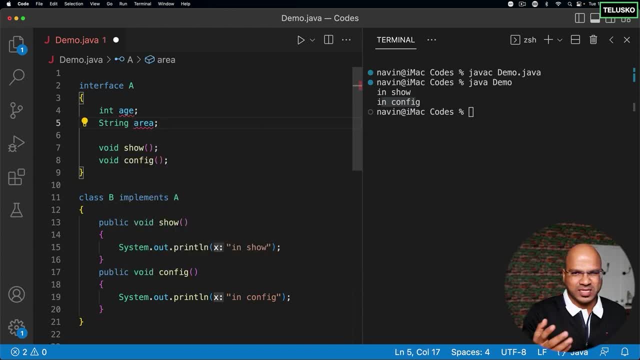 and let's say we have string area, so that's an area name, but you can see we got an error. that means can, I cannot create variables. that's weird. I just said we can right. so the only thing is every variable in the interface we can create actually those variables. the only thing is: 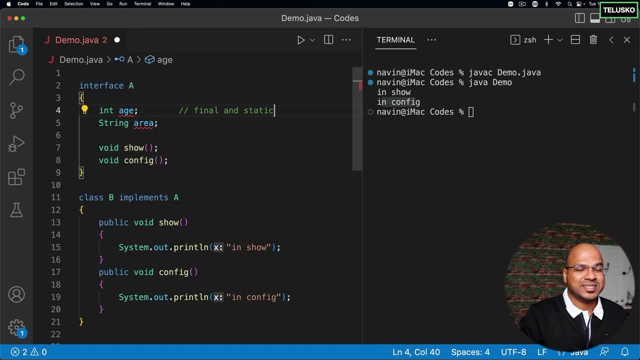 they are by default final variables and static. so all the variables inside the interface are by default final and static. okay, so that means we have to first initialize the variable. so when you say it's, it's final, we have to initialize the variable. right? okay, that's not my age, but let's say 44 and let's say area is. 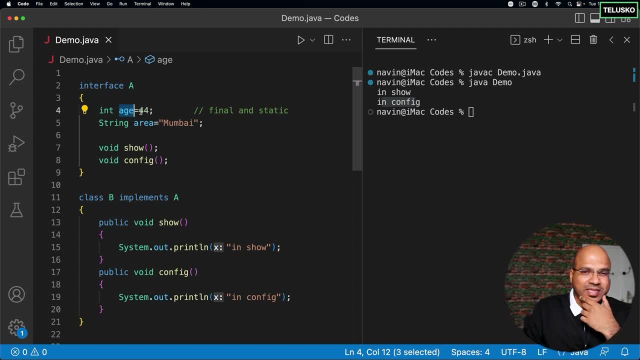 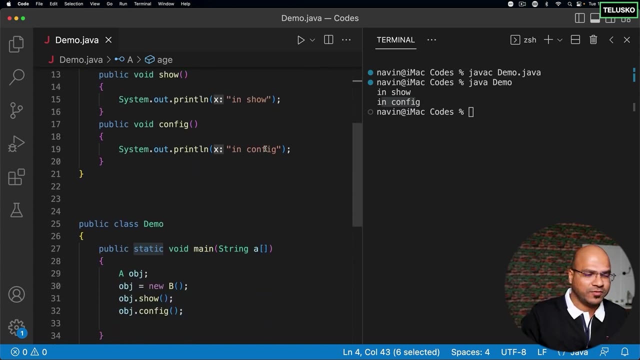 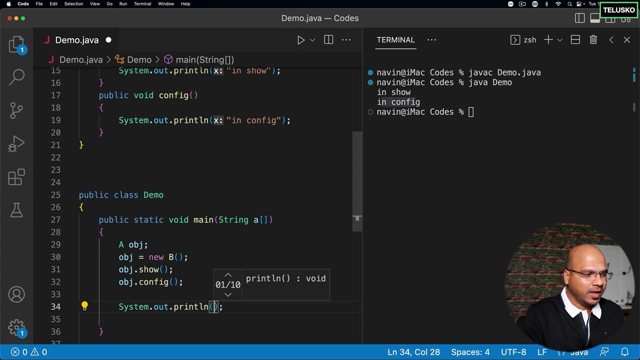 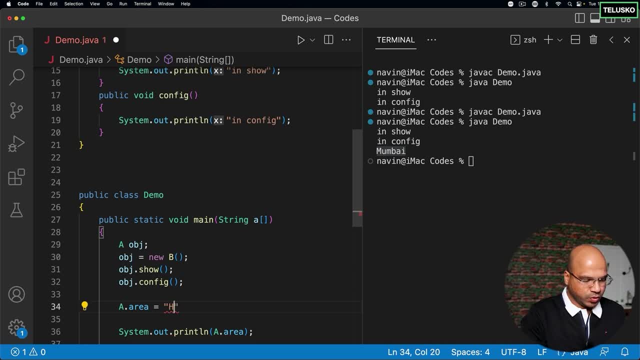 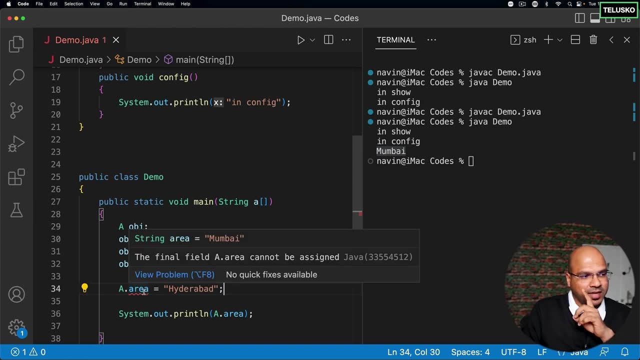 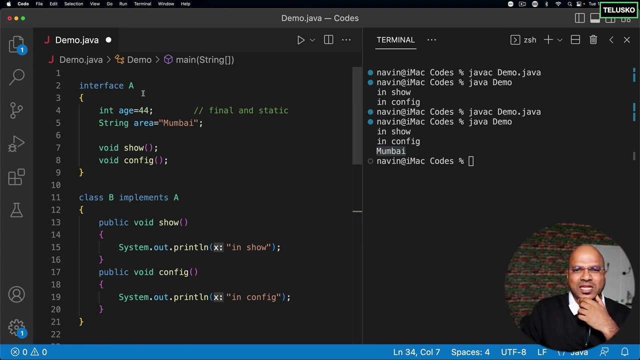